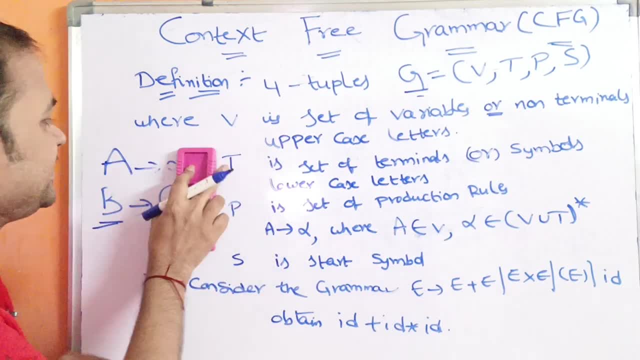 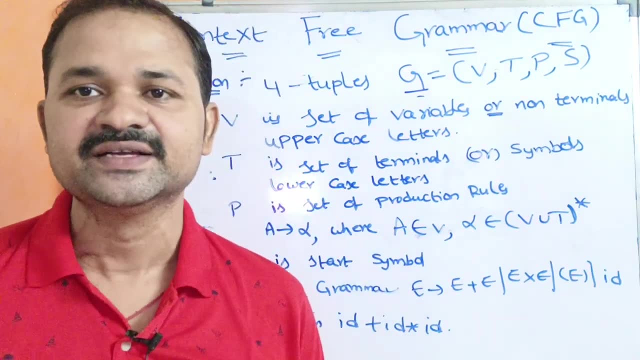 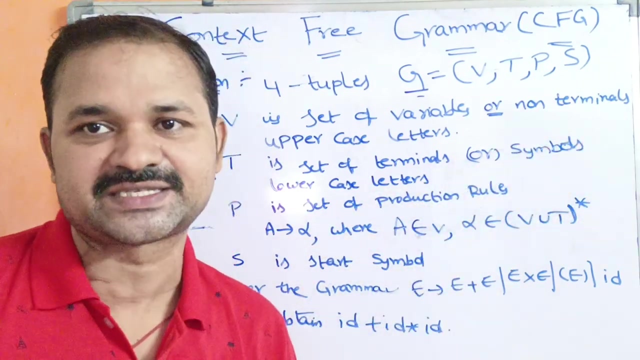 Now let us see the second tuple, That is T. T is a set of terminals, So T, the name itself specifies the mean. Now let us see The second tuple, that is T. T is a set of meaning. t stands for what? terminal symbols, or this can also be called as symbols. why? because 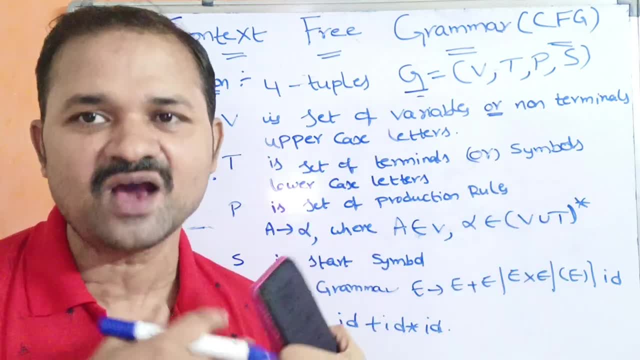 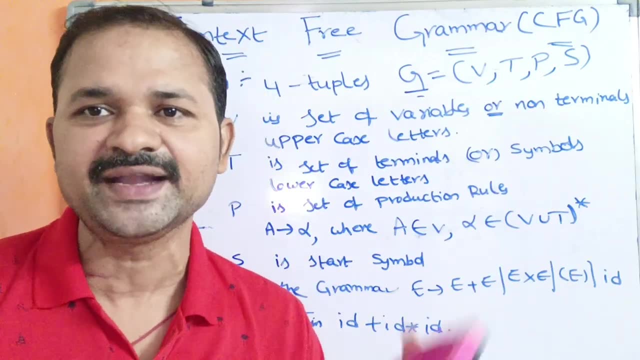 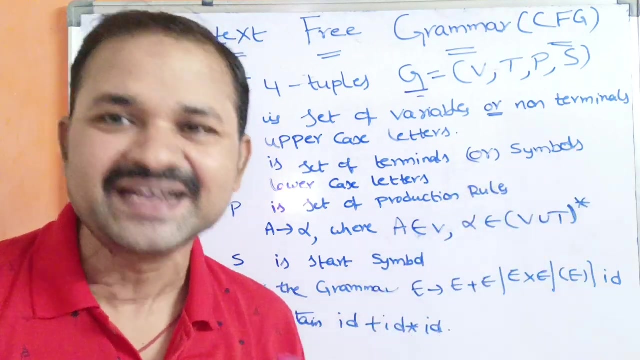 here we use symbols such as we can have several symbols, like left parenthesis, right parenthesis. the grammar may contains full stop, comma, digit plus minus star. likewise we can use n number of symbols and we can also use digits. also, we have digits from 0 to 9. we can use all those digits. 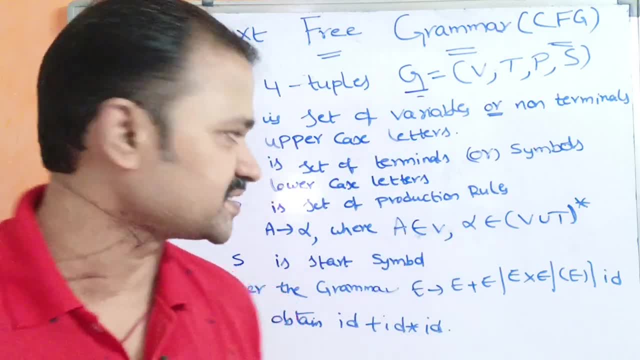 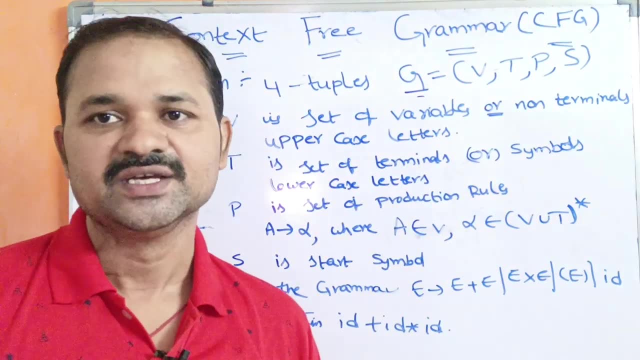 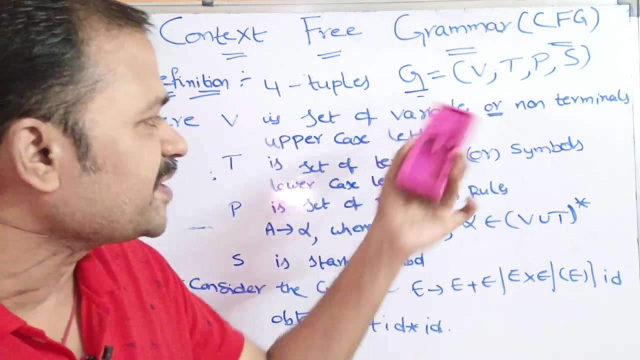 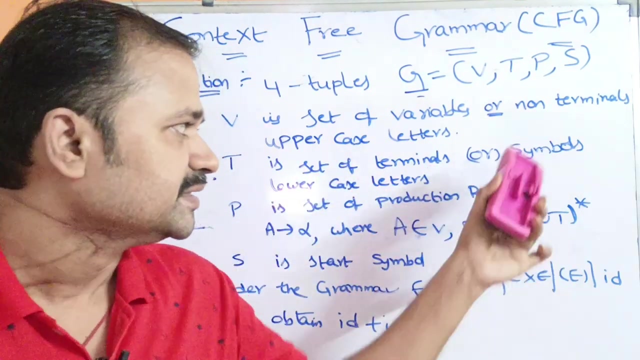 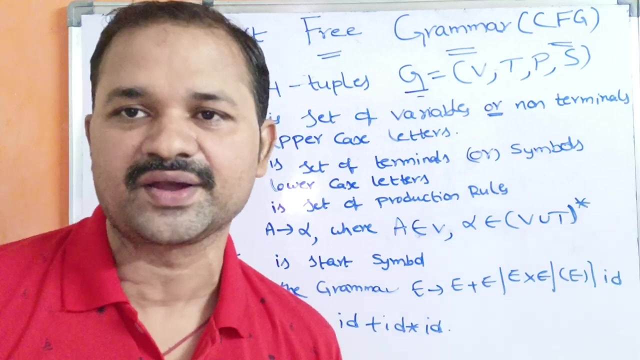 and combinations of digits, such as numbers, and in order to represent the terminals we use lower case letters, so terminals are always represented by lowercase letters. various variables are always represented by uppercase letters, so here terminals means lowercase letters or digits, numbers or symbols such as plus, minus, stars, so on. okay, here terminals are always useful. 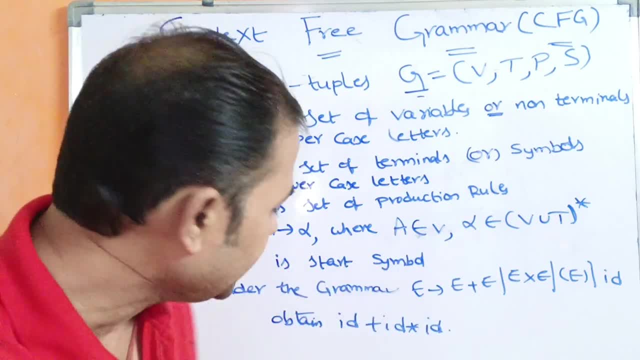 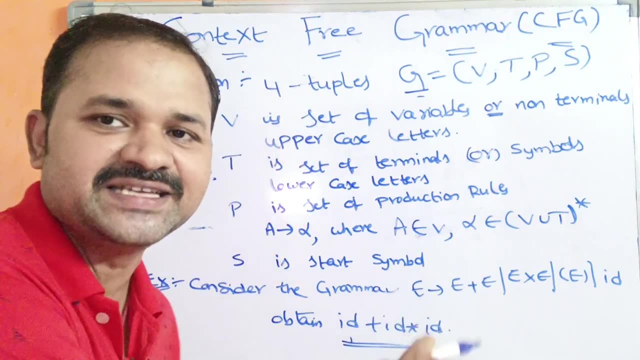 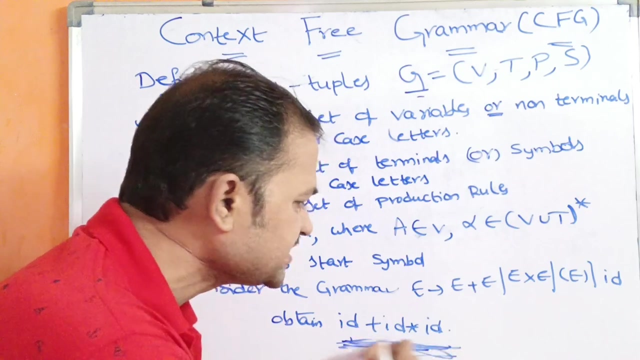 in order to derive a string here. let us see this example. here we have a grammar like this. here we want to generate the string id plus id, star id. so in our this is nothing but terminals. so terminals are always useful. here we are just adding a发 also for a acaba vehem, instead slowing down, but it is very useful. 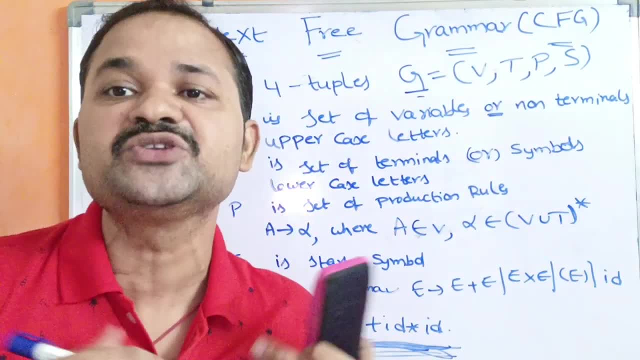 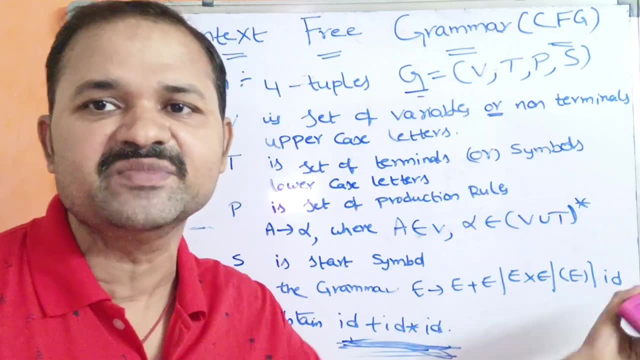 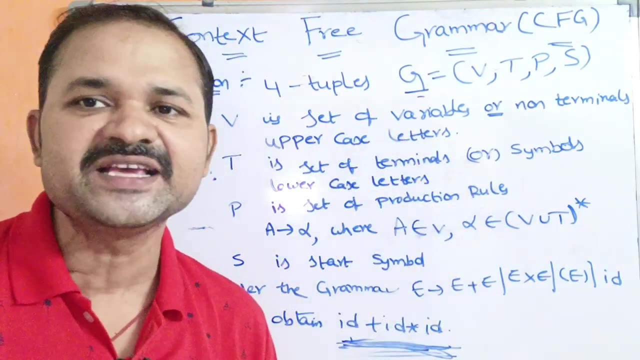 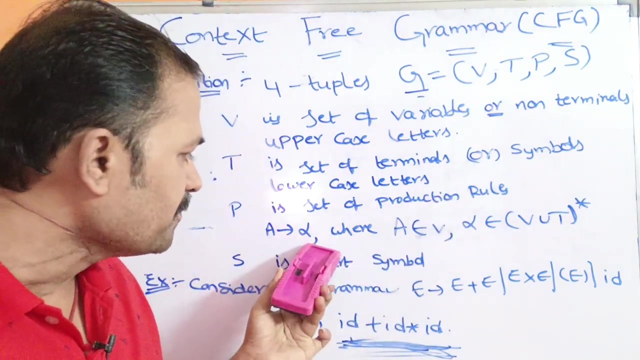 for generating the string. terminals are not used for substitution purpose, so in order to derive this thing, we have to use this, the terminals. this grammar contains a terminal called i. let us see the next one: p. p is a set of production rules, so p stands for production rule. here the production rule is of the form: a implies alpha, a produces alpha. where 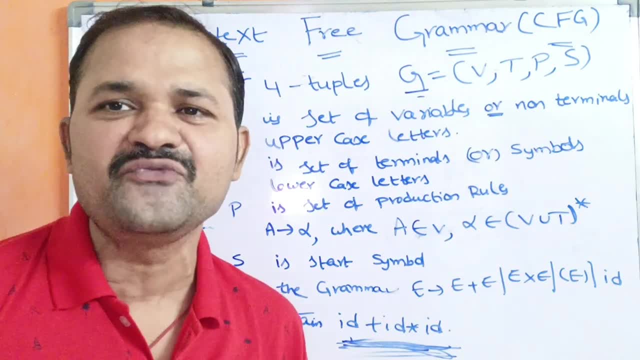 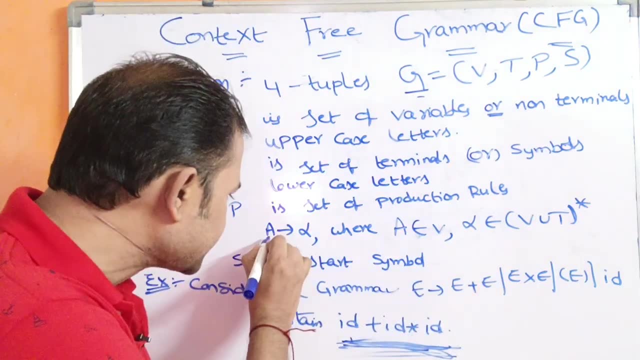 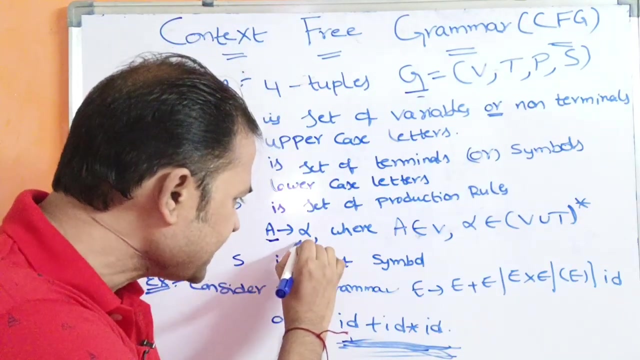 A belongs to V, So that means A is always a variable. A is always a non-terminal. This is left hand side. So A means A should always contains one non-terminal, One uppercase letter Variance. here the right hand side is alpha. 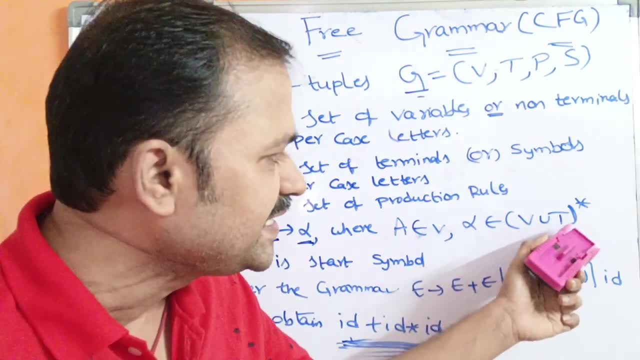 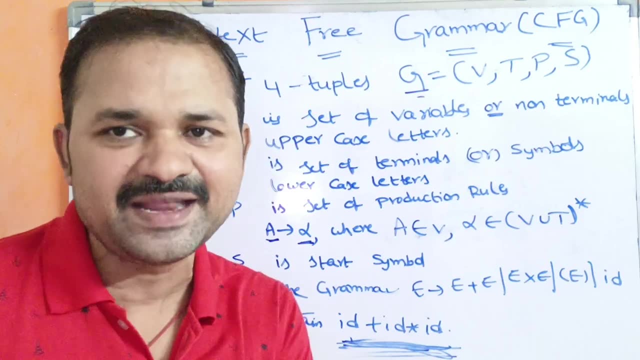 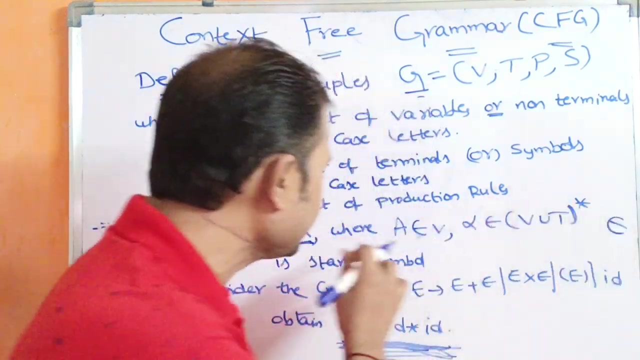 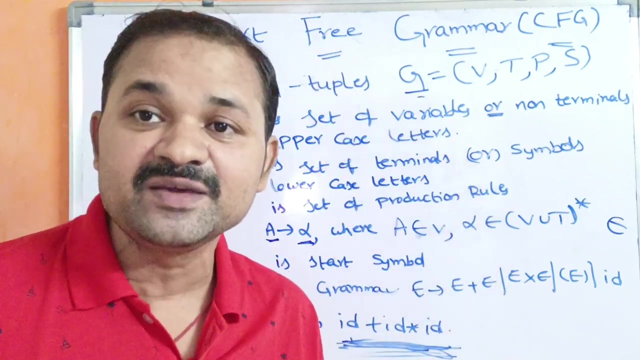 What is alpha? Alpha belongs to V union, T, whole star. So alpha is a combination of non-terminal and R-terminal Including zero occurrences. So zero occurrences means epsilon. So here in the right hand side we can have epsilon or we can have a combination of non-terminal and terminals. 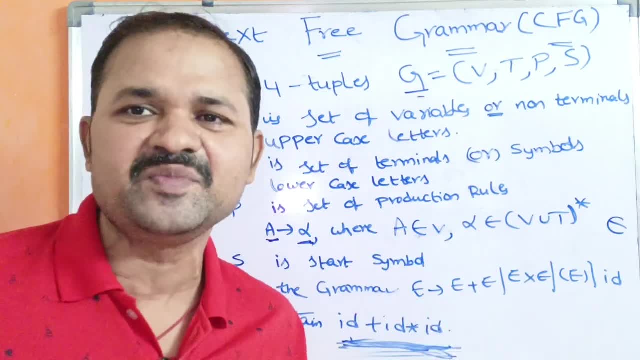 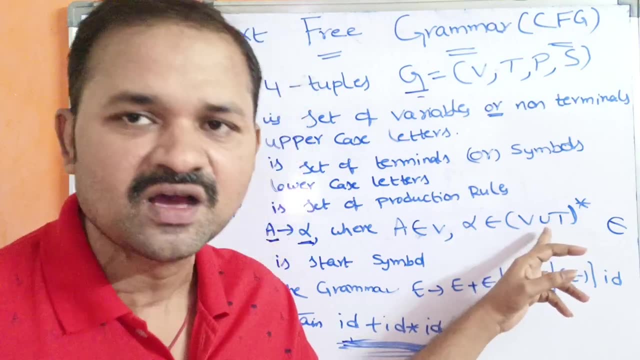 There is no problem. We can have both non-terminal and terminal, or we can have only non-terminal, or we can have only terminals. So there is no problem. Why? Because here we use R operator, So combination, And the last, Last one is S. 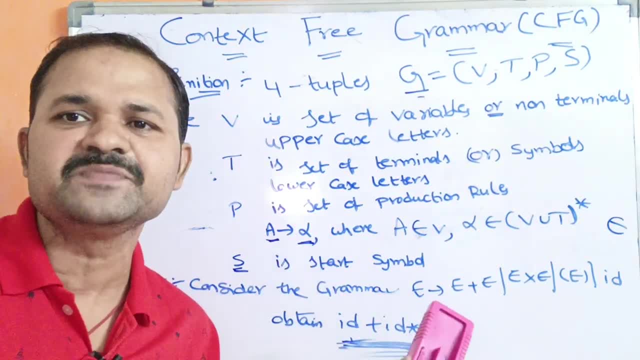 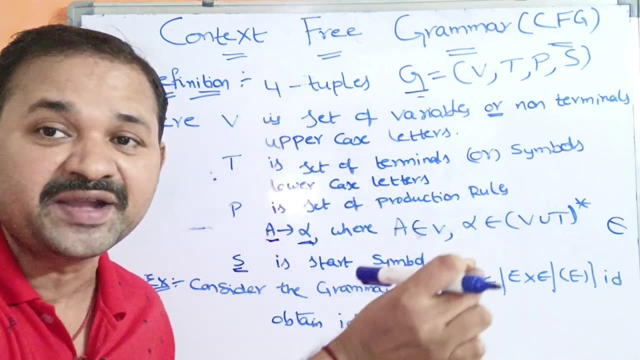 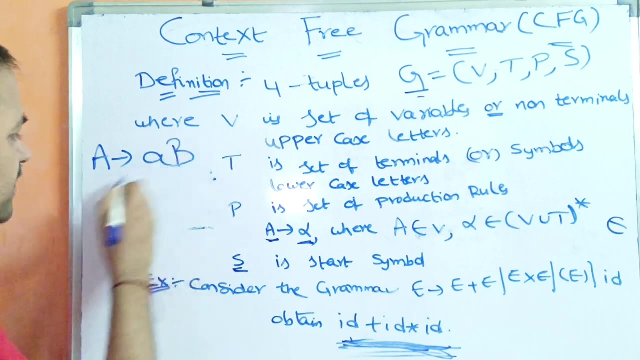 S is start symbol. Here. start symbol is always a non-terminal. Start symbol means the first two production left hand side- non-terminal. Let us see an example for this. Let we have productions like this: A implies AB, B implies CA. Next, C implies DE. 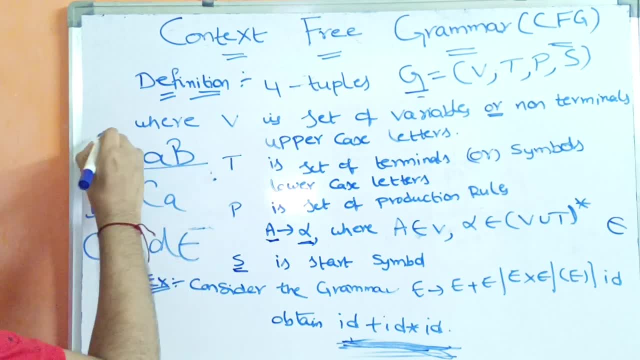 So here, what is the first two production? This is the first two production. What is First two production? left hand side A. So this A will become what Start symbol? Okay, So this is about the definition, The formal definition of the context, free grammar. 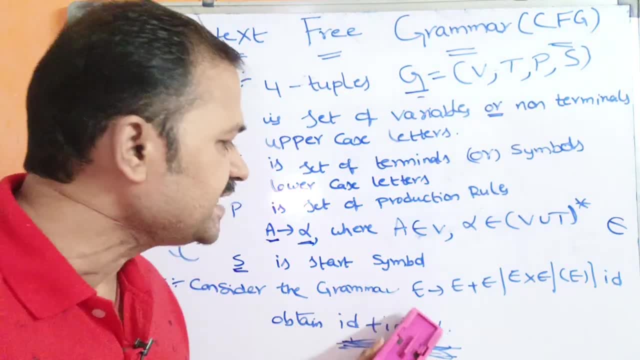 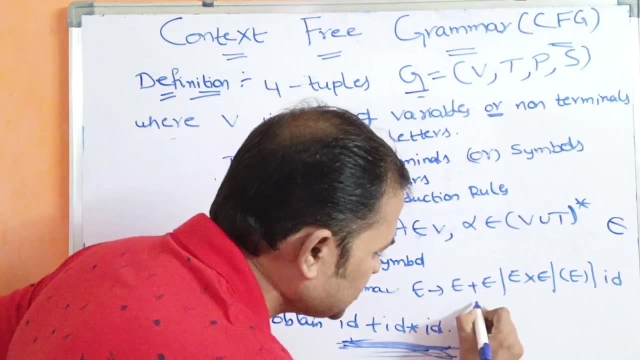 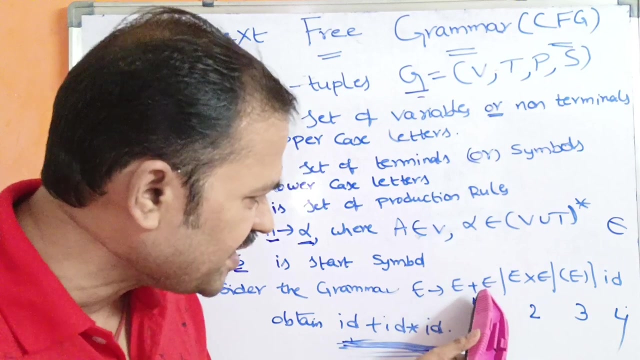 Now let us see an example for this. Consider the grammar: E produces E plus E R. So here E contains totally four productions. First, two production, Second production, Third production, Fourth production. Okay, So E produces E plus E. 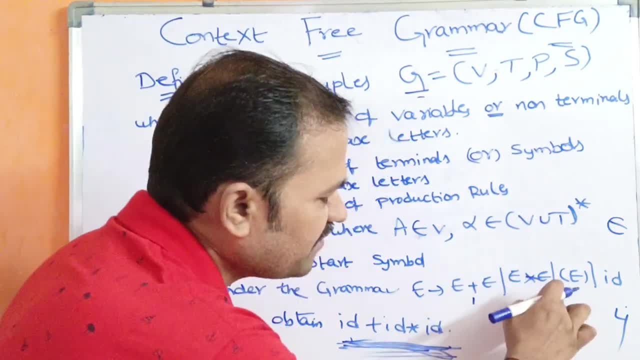 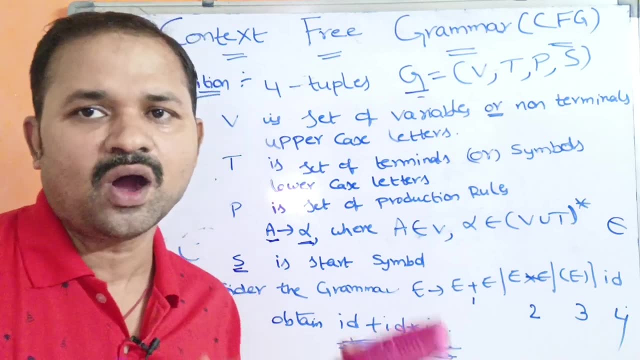 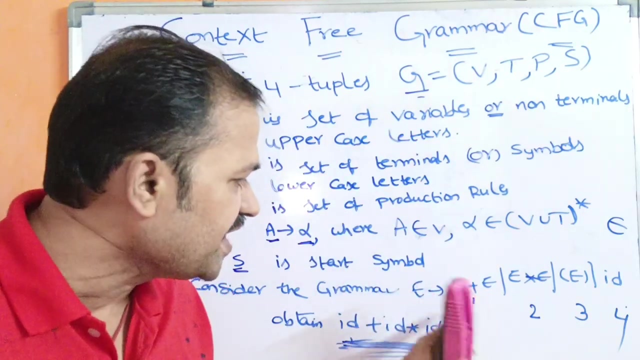 R, E, star, E R. Left parenthesis E, Right parenthesis E, R, I. So totally, here we have four productions. Now, in this grammar, what is B? What is B, B, T, P, S? B means non-terminal. Here we have only one non-terminal. 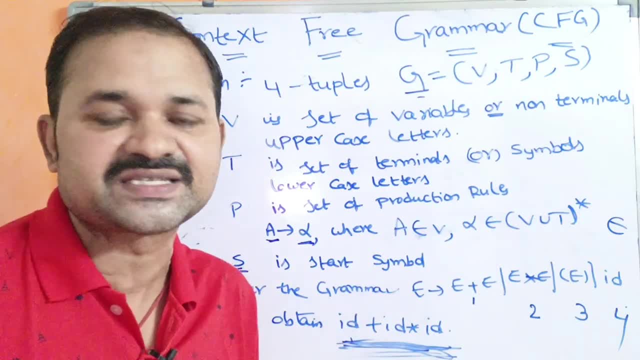 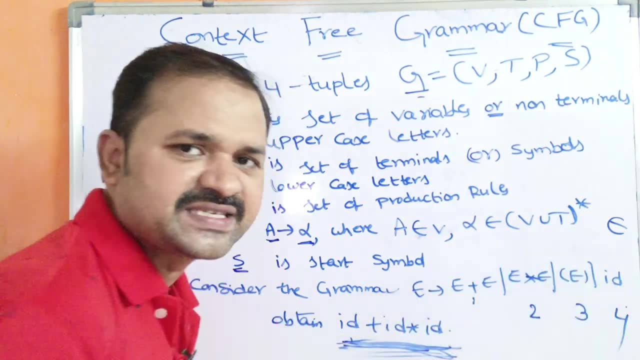 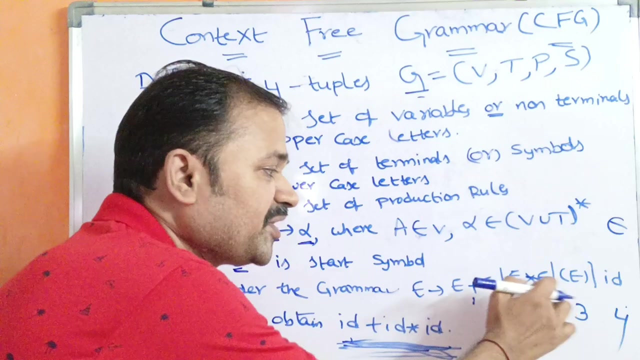 That is E And what is C. T means terminals. In this grammar we have terminals such as plus star, left parenthesis, right parenthesis, I, D, So all those are terminals, symbols. And what are the production rules? Totally we have four productions. are there? 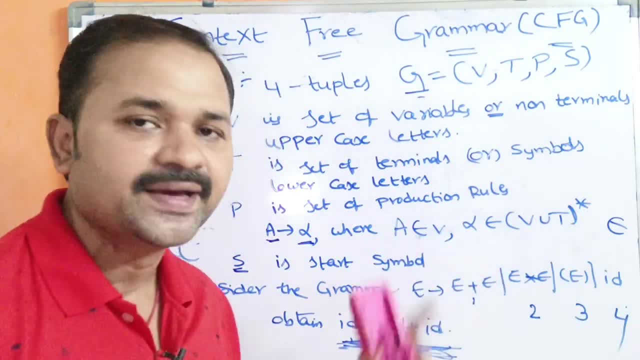 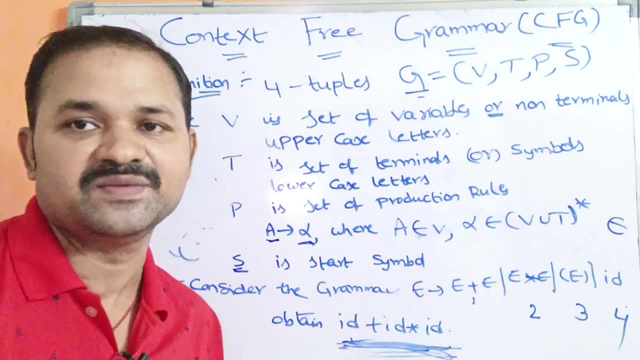 And what is the starting symbol Here? what is the first production? E produces E plus E. So the first production, left hand side, non-terminal, is E. So E is the start symbol Here. what is our target? Our target is: we want to obtain I D plus I D, star I D. 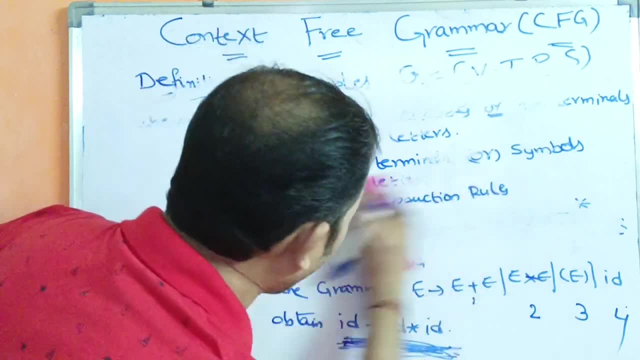 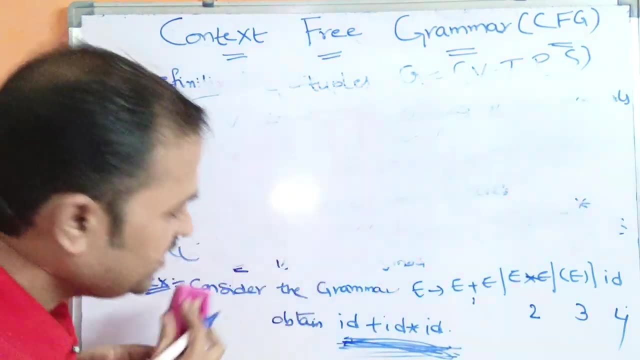 So this is an example. Now let us derive I D plus I D star I D. So I D plus I D star I D. So here we have a plus symbol. So that is why it is better to take the first production. 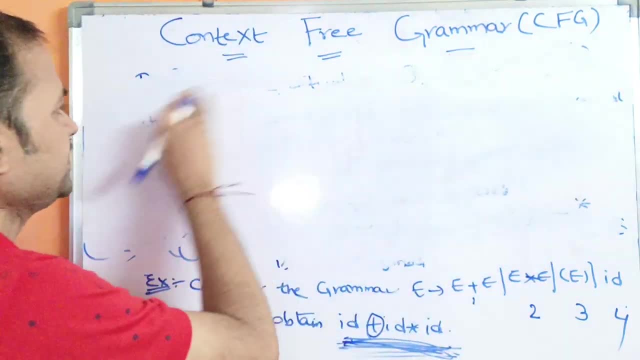 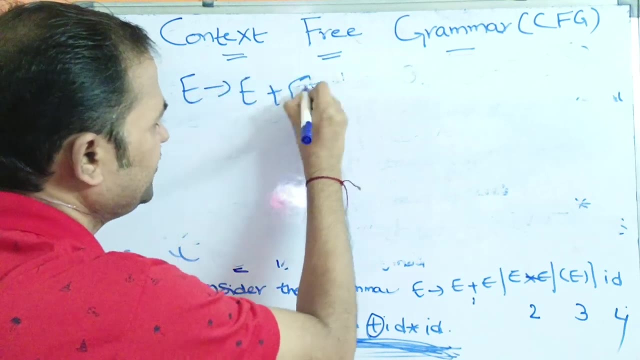 What is the first production? E produces E plus E. According to the choice, we can take any production: First or second, or third or fourth. E produces E plus E. This is the first production, Since E produces E plus E. Okay, 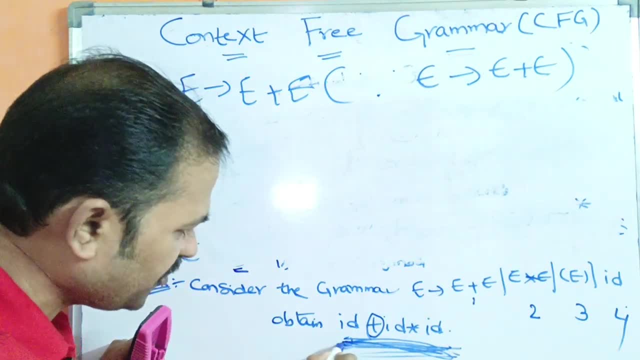 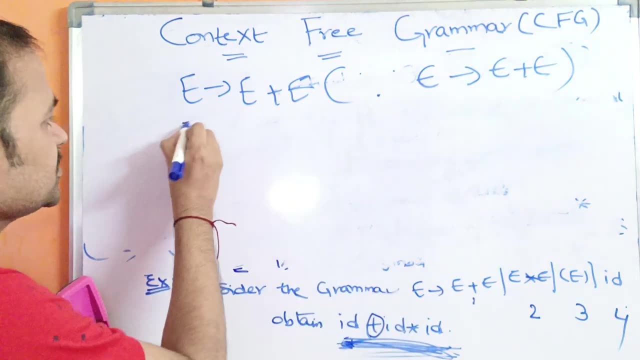 We have to derive First, we have to produce this I D. So here, from this E, we can get I D, From this E we can get I D star I D, So E produces. So let us produce I D. Why? Because we want to derive I D. 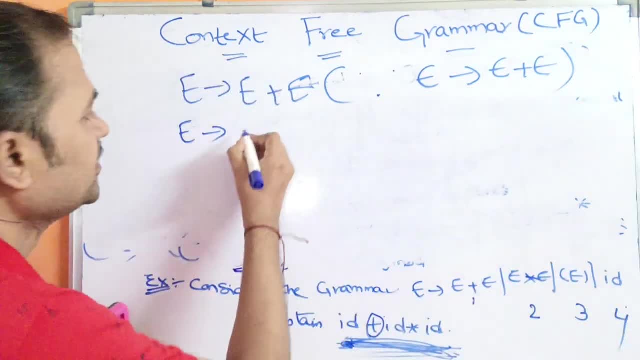 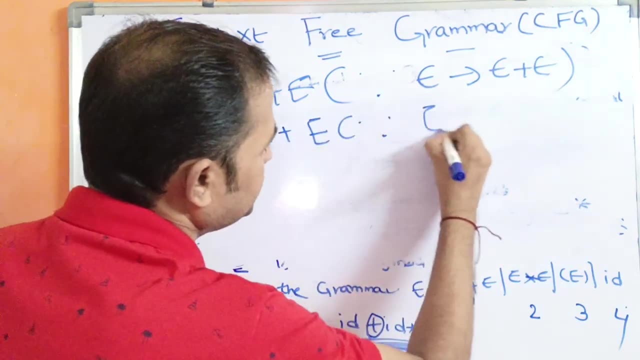 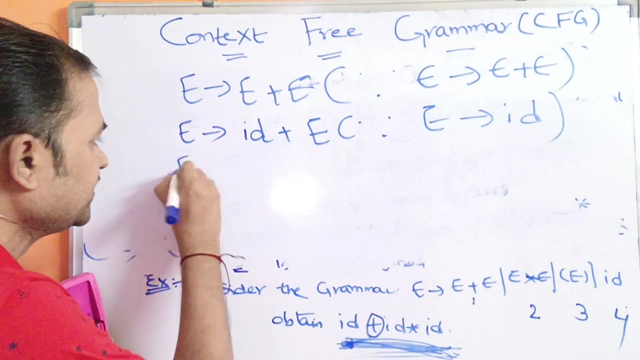 E produces. What is the first full production? I D, So I D plus E. So why we got I D? Why, Because E produces. I D is a production Which is Available in our grammar. Now let us see the next one. 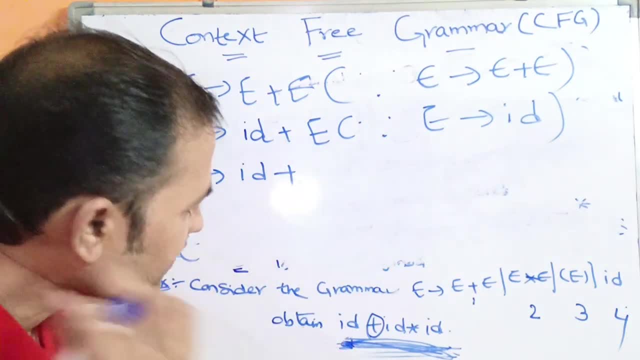 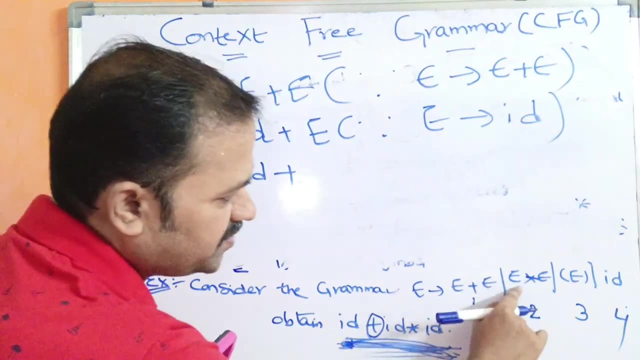 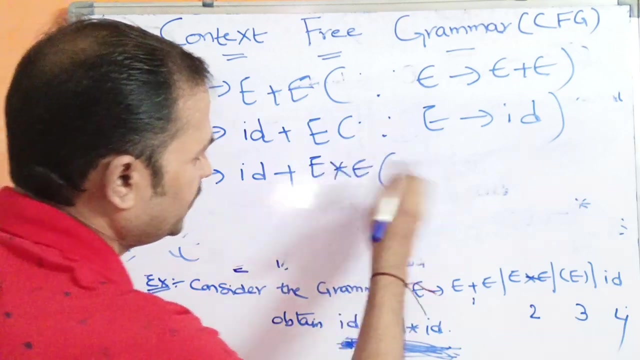 E produces I D plus E. So here we have to produces I D, star I D. So here we want to get star symbol. So star means here we have second production: E star E. So E star E, E star E. So why? because here we got E star E. 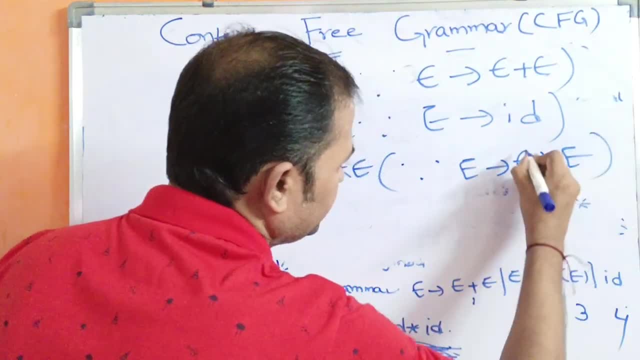 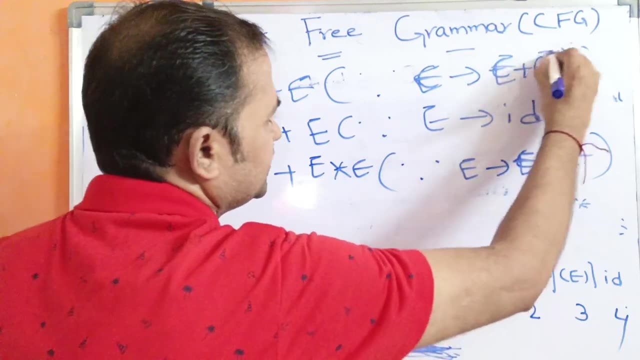 Because of second production. What is the second production? E produces E, star E. Here all are uppercase letters. only This is uppercase letter only. This is not epsilon. This is 0, only Ok. Next one: E produces I D plus. 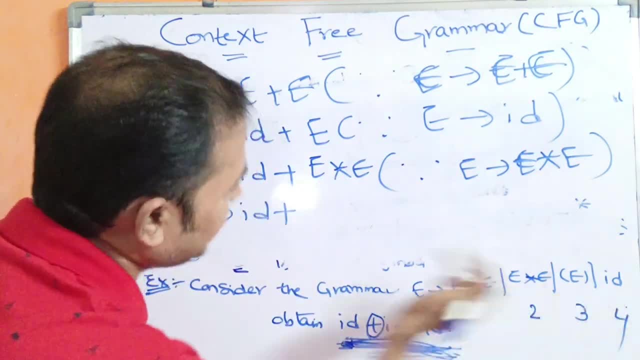 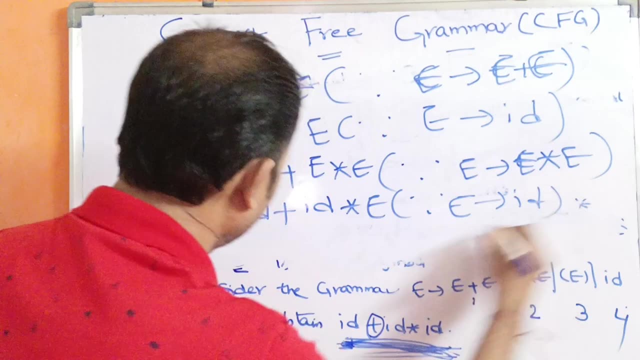 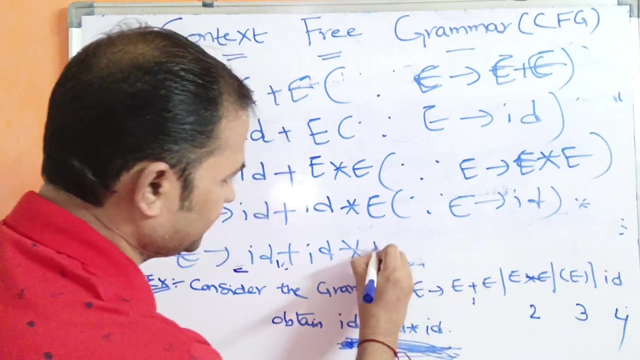 Next, here we have E From E we can get I D, So I D star E, Since E produces I D. Next one: E produces I D. plus, I D star From E we can get I D, So this is nothing but.